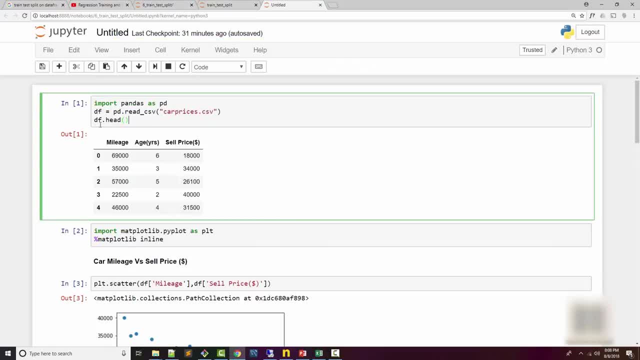 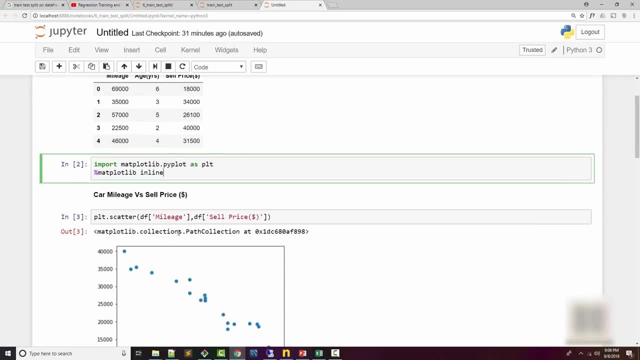 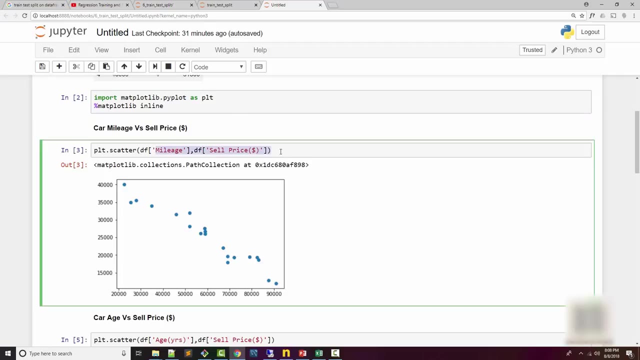 notebook. i have loaded this csv file into a data frame which looks like this, and then i'm using some matplotlib visualization to figure out the relationship between my dependent and independent variable. so here i have a plot of mileage versus the sell price and you can see a clear linear 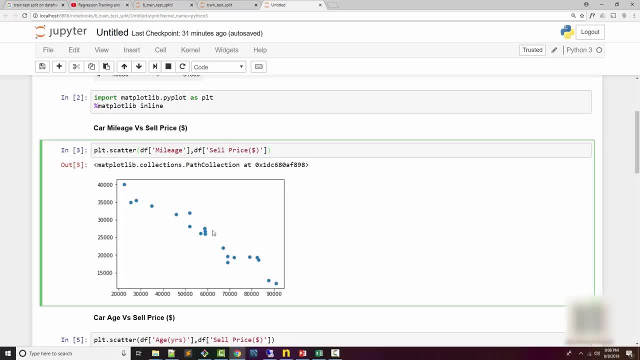 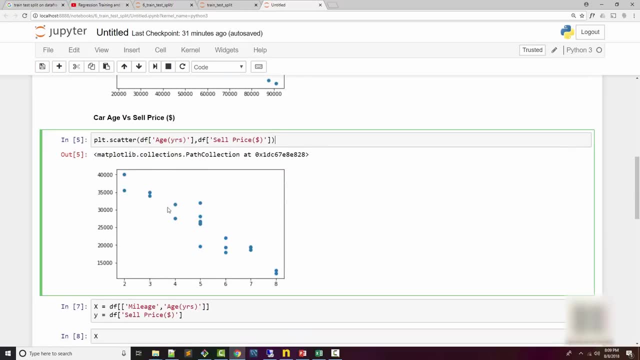 relationship. here we can draw a line that goes through all these data points. similarly for car age and sell price. i have plotted another scatter plot and here also you can sort of apply a linear relationship. so we are going to use a linear regression model. based on this visualization i have prepared my x. 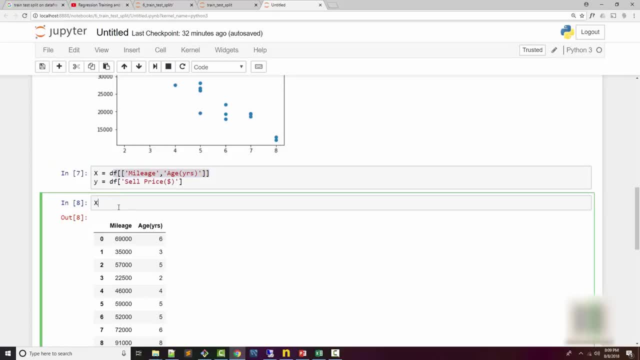 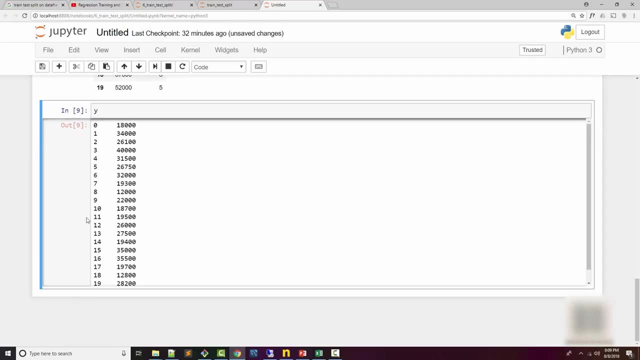 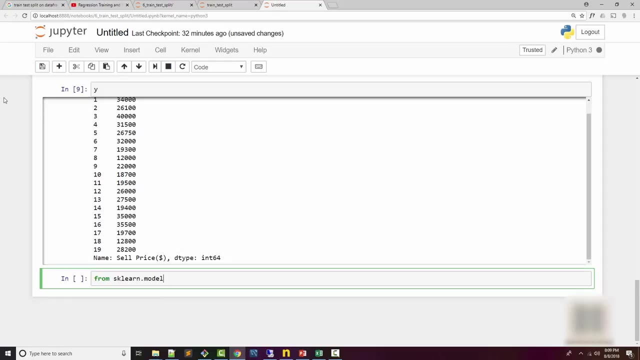 and y here. so x again mileage and age, and y is the selling price. the first thing we'll do here is: uh, use train test split method from sk, learn dot model selection. we are importing train test split method and then use this method, supply x and y as an input, and also you need to supply the ratio by. 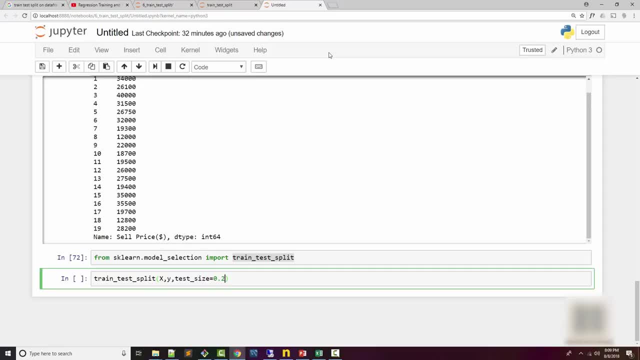 which you are splitting. so here i want my taste dataset size to be 20 and my training dataset size to be 80, so this is how you specify that. as a result, what you get is a x train dataset data set- why train and why taste. you get four parameters back, okay, and if you look at the length, 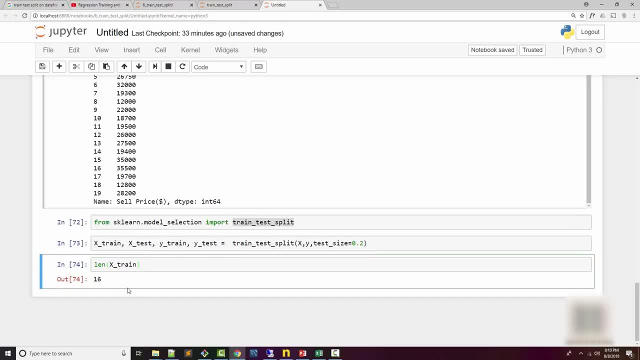 of whatever you got back. you will see it is 80 percent of your total data size. your total data size here is 20 and, based on 80 ratio, my training data set is 16 samples. amount of samples need to be 4 samples. look at taste and it will be 4, as you would expect it to be. so 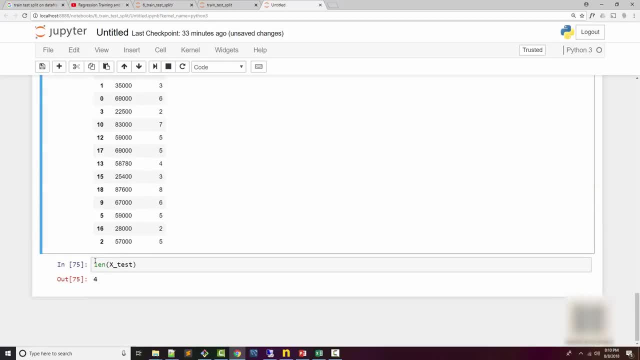 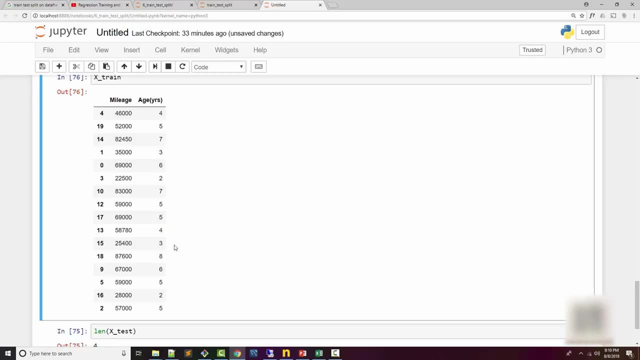 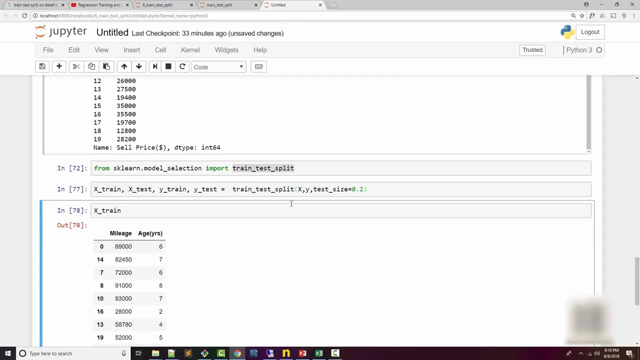 if you check the actual content of your x train, you will see that it choose the random samples. it's not selecting the first 80 percent of the samples, just using random samples, which is good. if you execute this method again and again, you will see that the the samples will change here. 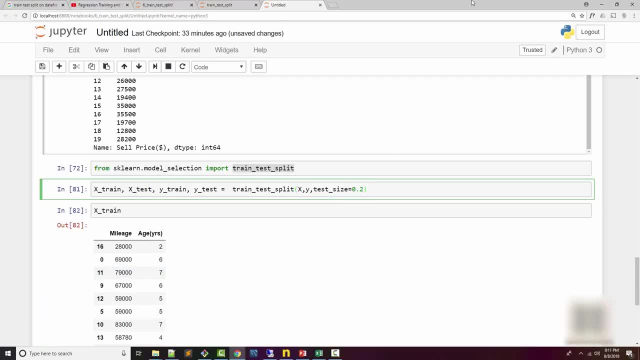 now, sometimes you want your sample to remain same and for that you can use this random state method. if you use random state, remember it's gonna use same samples, okay? so for random states, value of 10, it will always produce the same output. you can see that my x train is not changing now, right? 22? 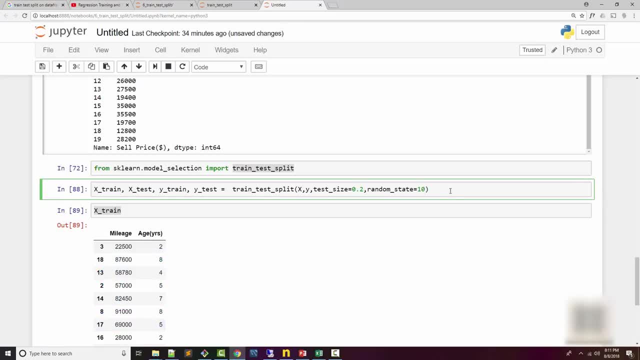 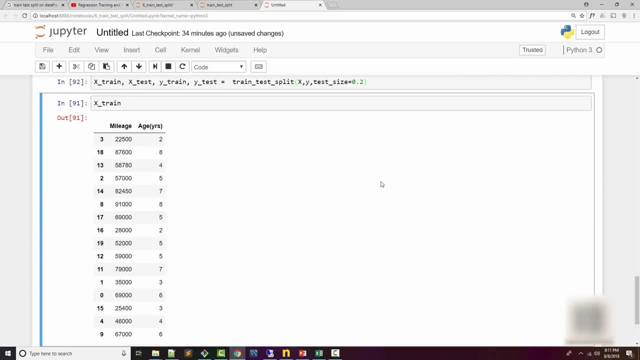 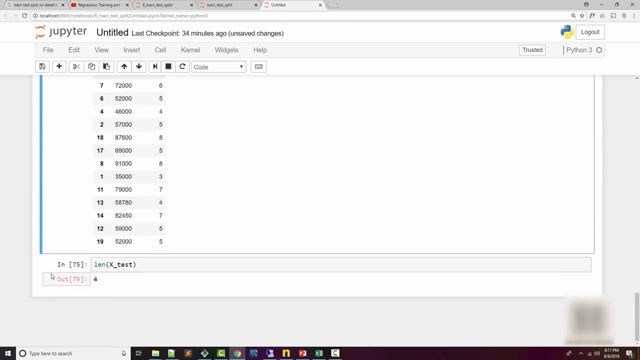 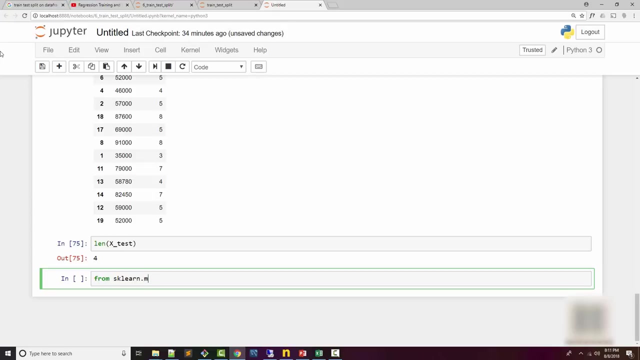 500. you'll see these values are not changing when i execute this multiple times, whereas if i didn't have this parameter, it was changing all the time. so if you do ctrl enter, you can see that right. okay, now let's use our linear regression model, so you can guess that i am going to import linear regression class. 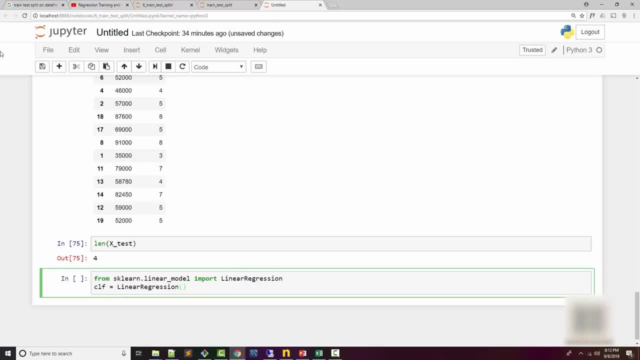 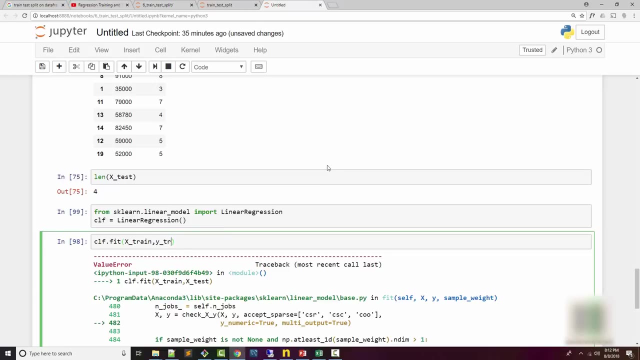 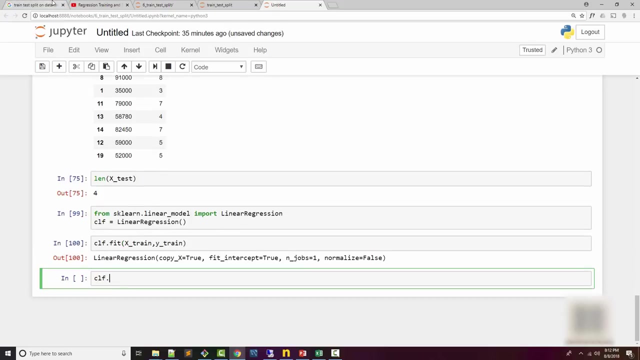 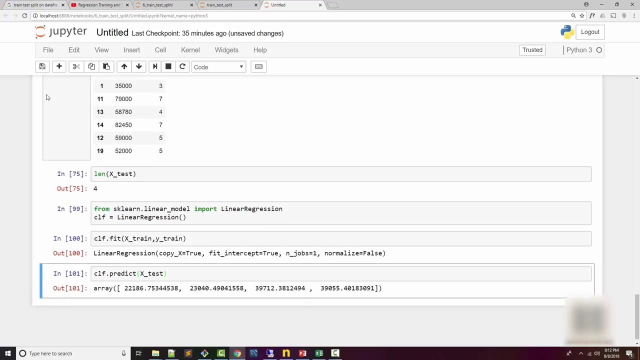 and create my classifier, which is nothing but an object of this class, and then you use a fit method to actually train your model. okay, so i need to use x train, y train and my model is trained now. and now i can uh call predict method on my actual test data set. so my model is pretty predicting. 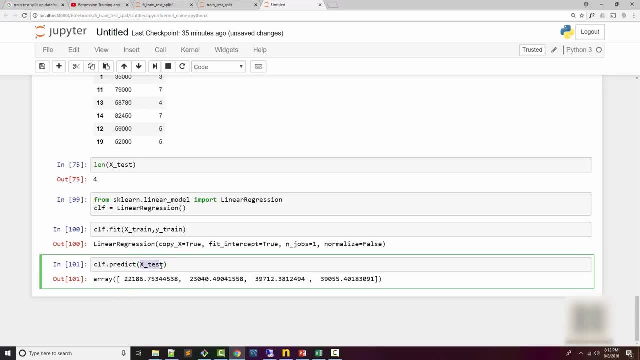 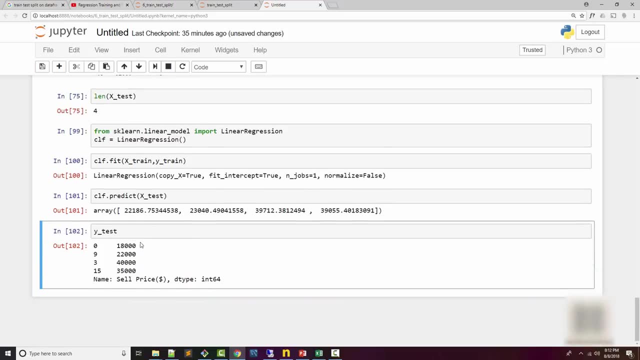 that the values are going to be the same. or the values are going to be the same, or the values are, uh, predicted values for my x test are these? let's look at how my y taste looks. so my y test looks like this. so values are kind of in similar range, but not exactly. so let's check. 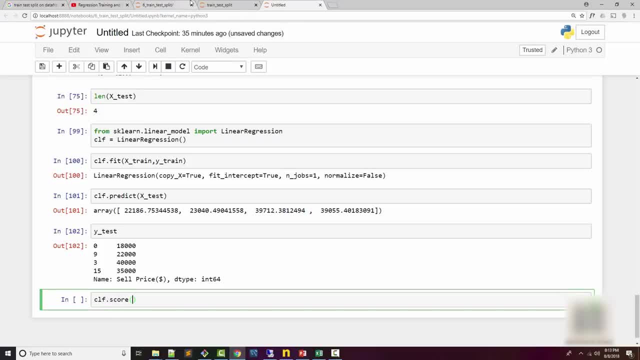 the accuracy of the model by calling score method. so what score method will do is it will use x test and predict these values and then compare it against these y test values and tell you the accuracy. so here accuracy is 0.89 percent. okay, that's just because of the nature of my data set. 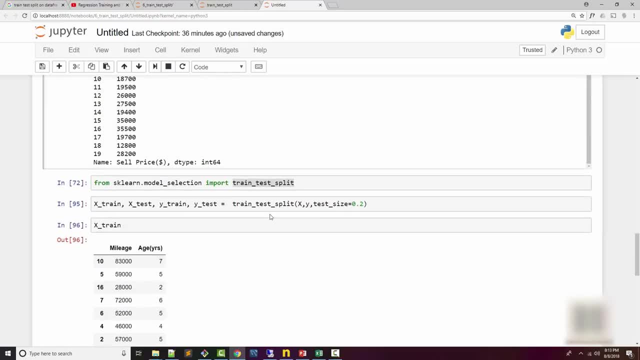 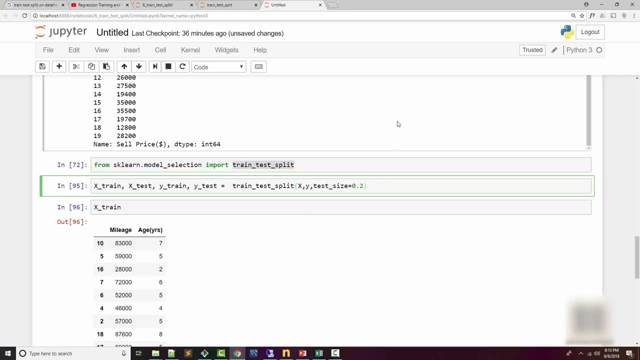 but that's all i had for this tutorial. uh, you learned that how train test split can be used to split your actual data set so you can change your percentage ratio between the two data set by modification this. if I do this, then it will be 70: 30 ratio. okay, so that's all I had for this.